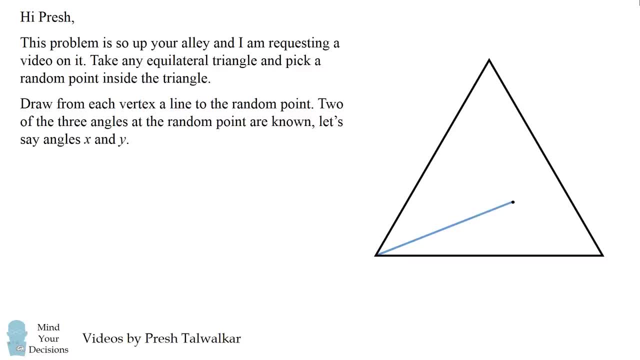 Draw from each vertex a line to the random point. Two of the three angles at the random point are known, Let's say angles X and Y. If the three line segments from each vertex to the random point were removed out of the original triangle to form a new triangle, 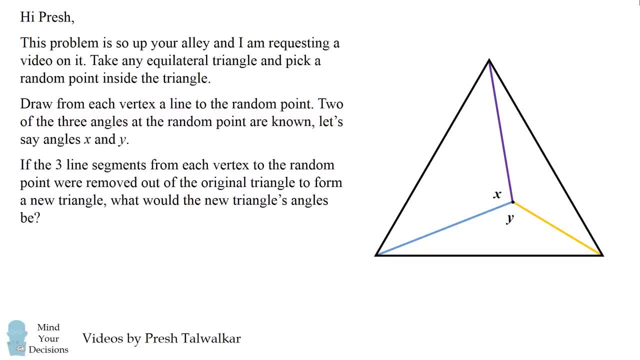 what would the new triangle's angles be? Try to figure it out. I was unable to do so, but I do have the unbelievable solution if you have any trouble. Regards Daniel E. Now I will say I did give this problem an honest effort and I was stumped. 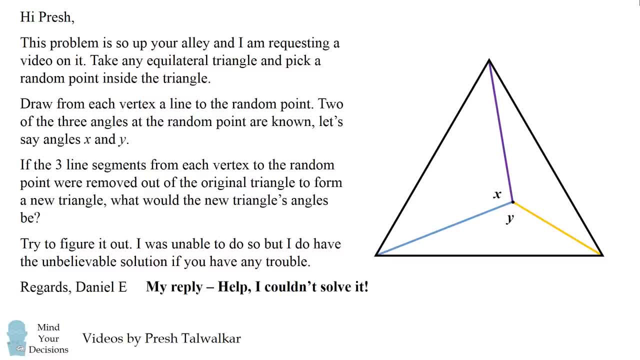 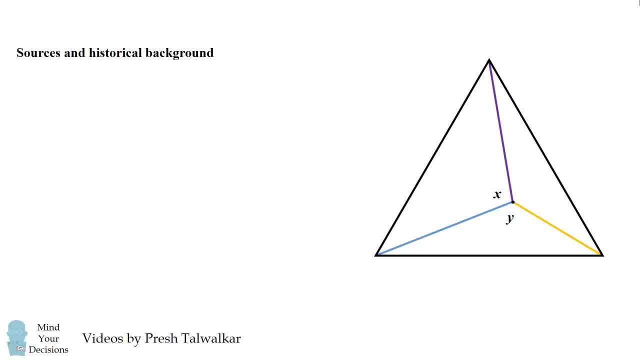 Please help me solve this problem. Daniel then provided me with the solution. This problem also has an interesting background. There's a lot more about it in the video Simple Math Problems to Fool the World. You can find all the best on the YouTube channel: Gold-Plated Goof. 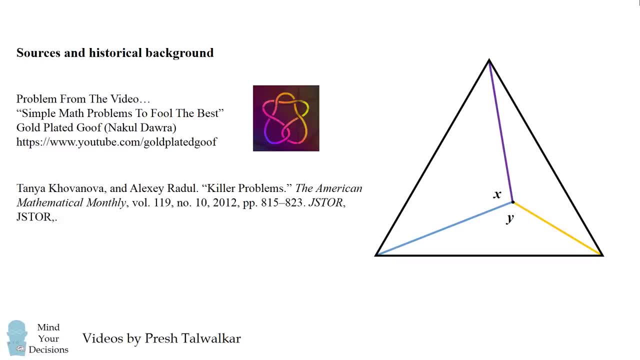 The problem is also part of a collection of quote killer problems that were very easy to state and almost impossible to solve unless you knew a very specific trick. As such, these problems could be used for discriminatory purposes at universities. So please check out these sources for more about the historical background about this problem. 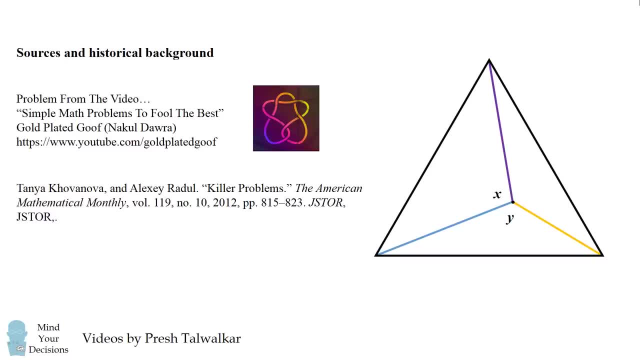 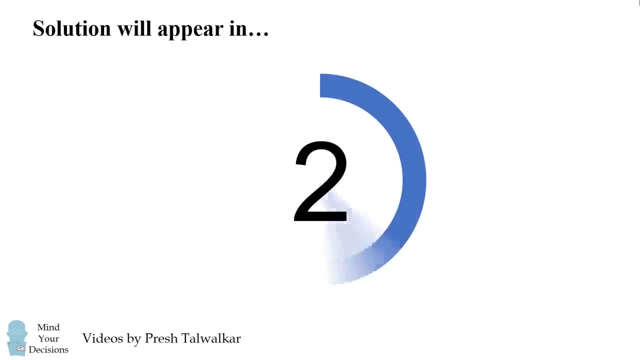 and other problems. In this video I'm just going to focus on the problem and show you the solution. So can you figure it out? Give this problem a try and, when you're ready, keep watching the video for the solution. So preliminary to get started is: 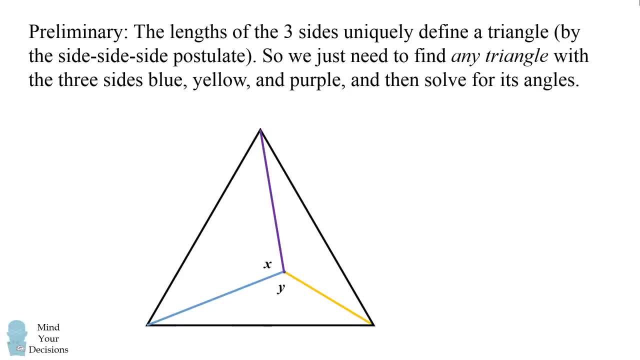 that the lengths of the three sides uniquely define a triangle. by the size of the triangle. This is called the side-side-side postulate. So we just need to find any triangle with the three sides blue, yellow and purple and then solve for its angles. 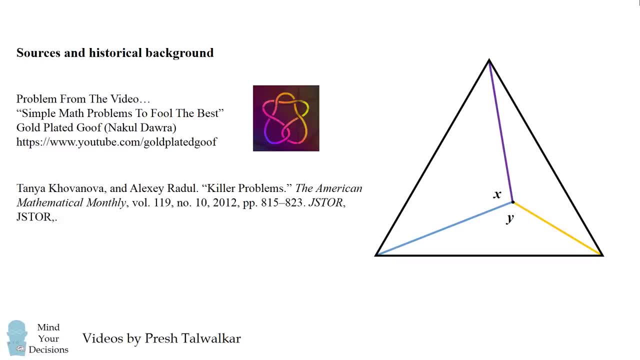 The problem is also part of a collection of quote killer problems that were very easy to state and almost impossible to solve unless you knew a very specific trick and, as such, these problems could be used for discriminatory purposes at universities. So please check out these sources for more about the historical background about this problem. 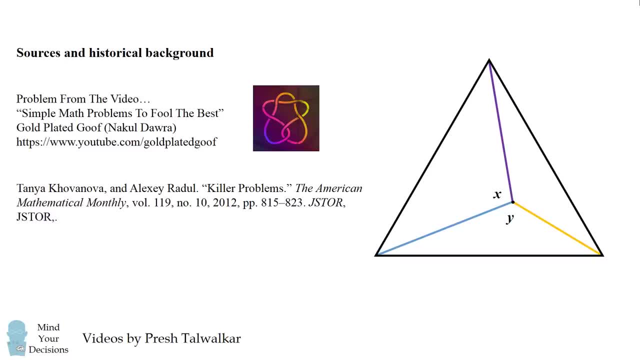 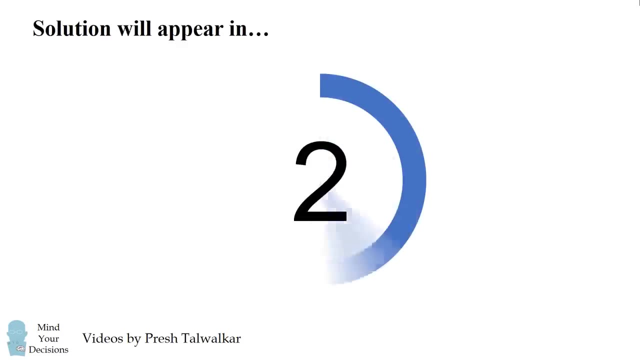 and other problems. In this video I'm just going to focus on the problem and show you the solution. So can you figure it out? Give this problem a try and, when you're ready, keep watching the video for the solution. So preliminary to get started is: 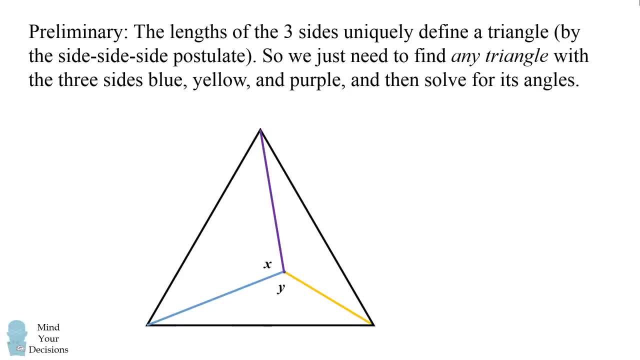 that the lengths of the three sides uniquely define a triangle. by the side of the triangle, This is called the side-side-side postulate. So we just need to find any triangle with the three sides blue, yellow and purple and then solve for its angles. 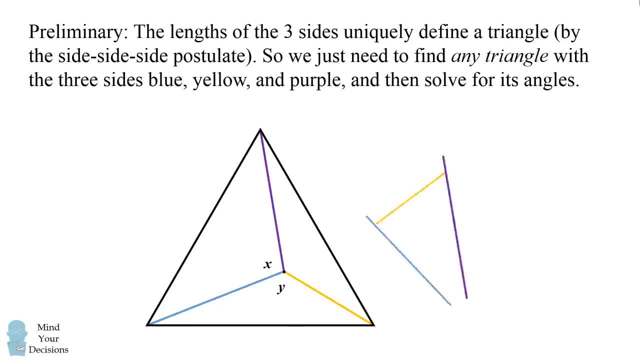 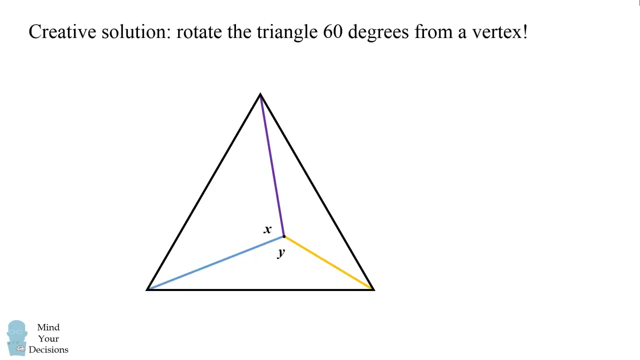 So how do we do that? It seems pretty impossible. How can we get from this triangle's angles to the original angles? Well, let me present to you the ingenious trick. The problem becomes easy if you rotate the triangle 60 degrees from a vertex. 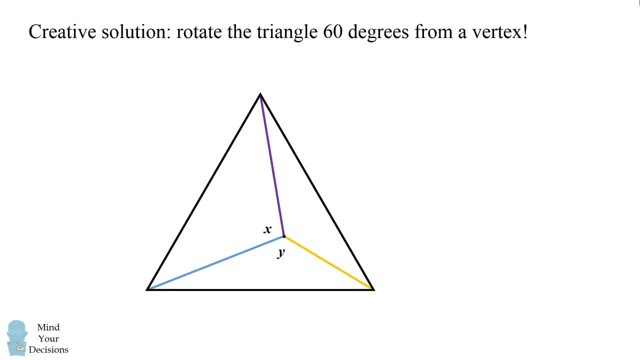 So let's imagine rotating this triangle 60 degrees counterclockwise from the bottom left vertex. We now connect the random point on the rotated triangle to the original angle And we will show that we have now found a triangle with a blue, yellow and purple side. 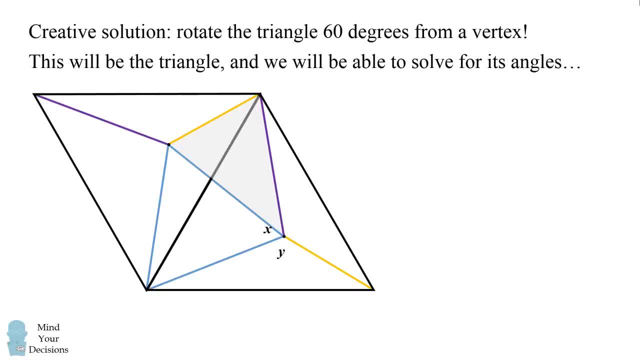 So this will be the triangle and we will be able to solve for its angles. So that's going to be the plan of the proof. Now, how do we know? this is the particular triangle we're looking for. So let's work each step out. 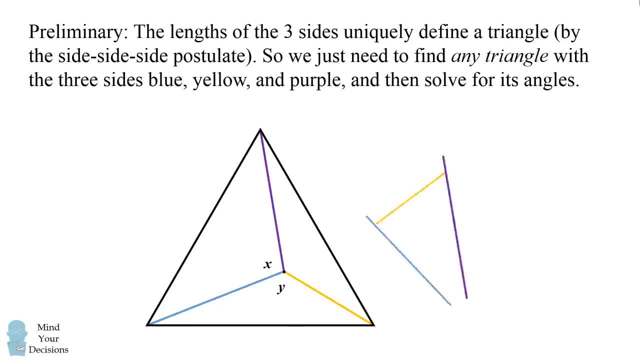 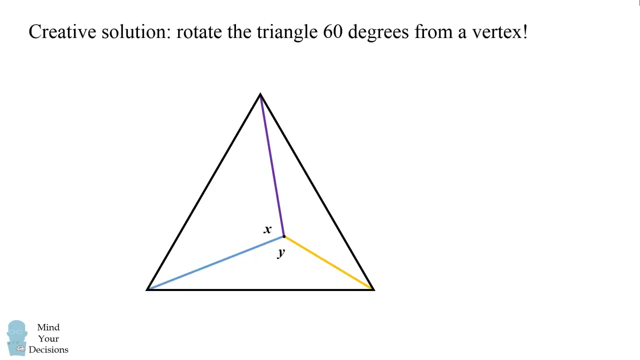 So how do we do that? It seems pretty impossible. How can we get from this triangle's angles to the original angles? Well, let me present to you the ingenious trick. The problem becomes easy if you rotate the triangle 60 degrees from a vertex. 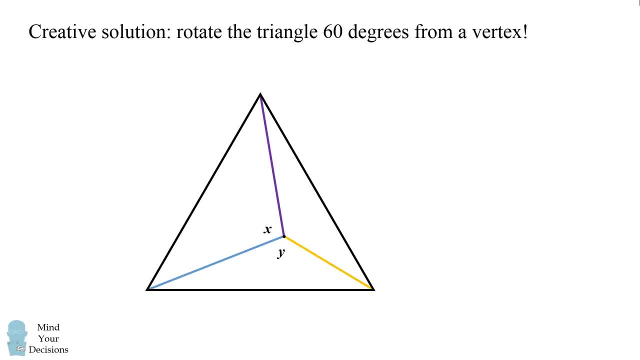 So let's imagine rotating this triangle 60 degrees counterclockwise from the bottom left vertex. We now connect the random point on the rotated triangle to the original angle. We now connect the random point on the rotated triangle to the original angle. We now connect the random point on the rotated triangle to the original angle. 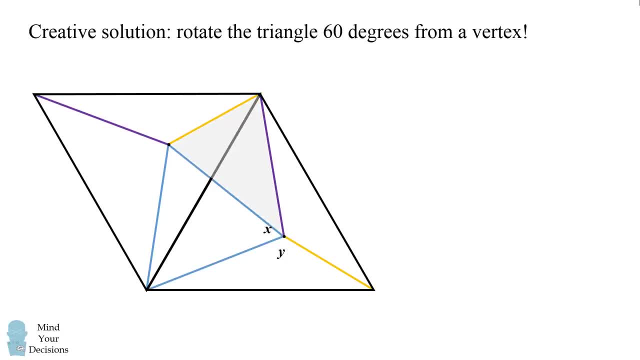 And we will show that we have now found a triangle with a blue, yellow and purple side. So THIS will be the triangle and we will be able to solve for its angles. So that's going to be the plan of the proof. Now, how do we know? this is the particular triangle we're looking for. 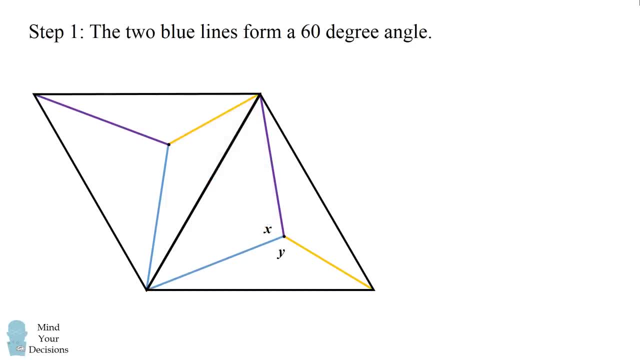 So let's work each step out. The first step is that the two blue lines. The first step is that the two blue lines form a 60 degree angle. This is because the triangle was rotated 60 degrees. but just to be sure we know, this is a 60 degree angle. 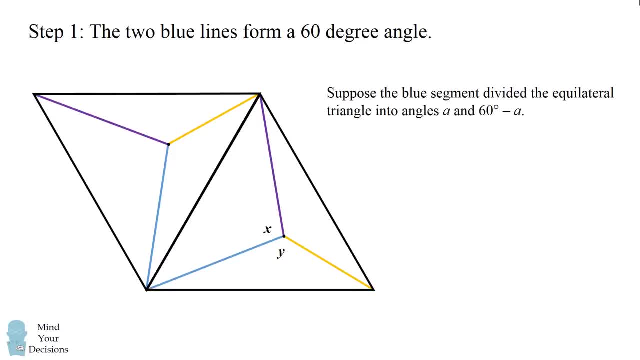 let's figure it out. Suppose the blue segment divided the equilateral triangle into angles A and 60 minus A. We'll mark the same angles in the triangle that was rotated. Now the two blue lines make an angle of 60 minus A plus A, which is 60 degrees. 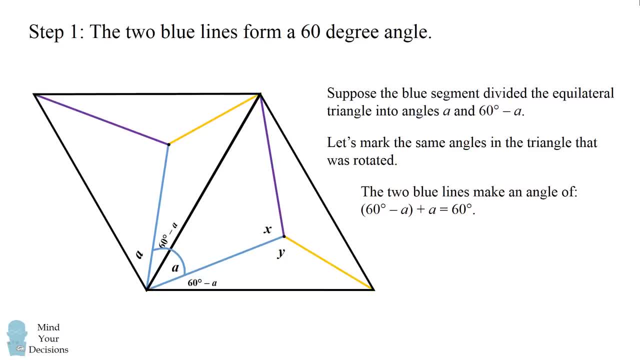 So we've proved that this angle between the two blue lines is 60 degrees. Next, we'll show that the blue lines define an equilateral triangle. We'll form a triangle by connecting the endpoints of the two blue line segments. The two blue line segments have the same length. 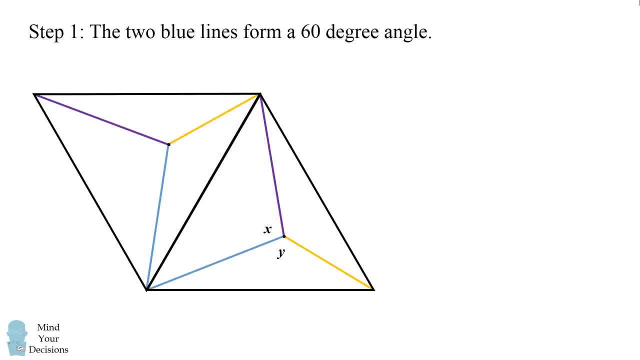 The first step is that the two angles are the same. The two blue lines form a 60 degree angle. This is because the triangle was rotated 60 degrees. But just to be sure we know this is a 60 degree angle. let's figure it out. 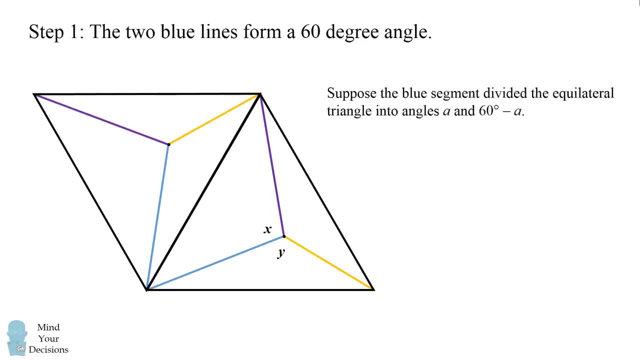 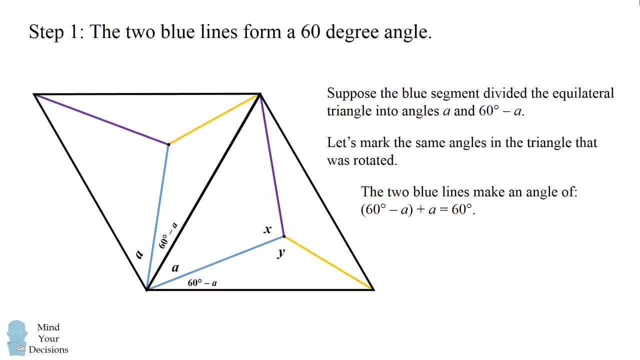 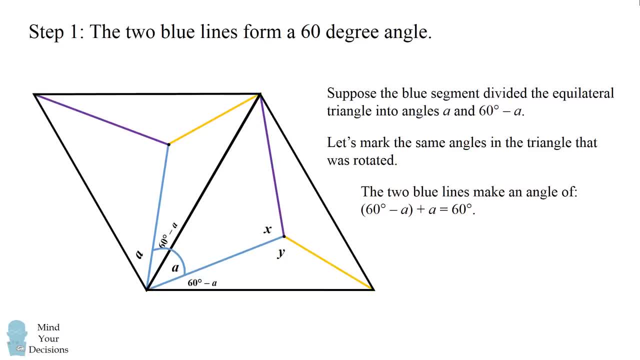 So we've proved that this angle between the two blue lines is 60 degrees. Next, we'll show that the blue lines define an equilateral triangle. We'll form a triangle by connecting the endpoints of the two blue line segments. The two blue line segments have the same length. 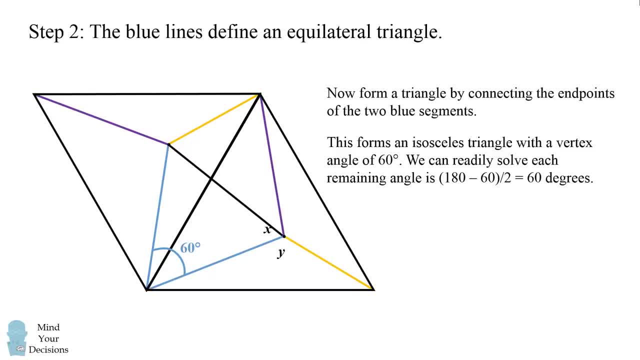 Therefore, we have an isosceles triangle with a vertex angle of 60 degrees. Therefore, we have an isosceles triangle with a vertex angle of 60 degrees. Therefore, we have an isosceles triangle with a vertex angle of 60 degrees. 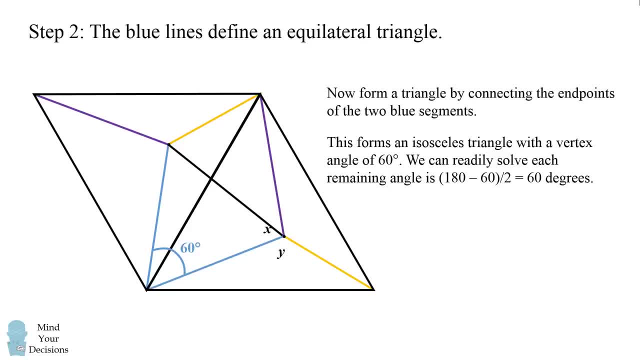 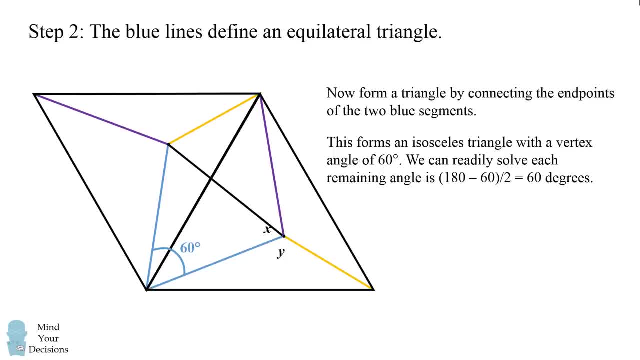 The remaining two angles will be equal to each other, and the sum of the three angles in a triangle is 180 degrees. So each remaining angle will be 180 minus 60, and then we divide that by 2.. So each remaining angle will be 180 minus 60, and then we divide that by 2.. 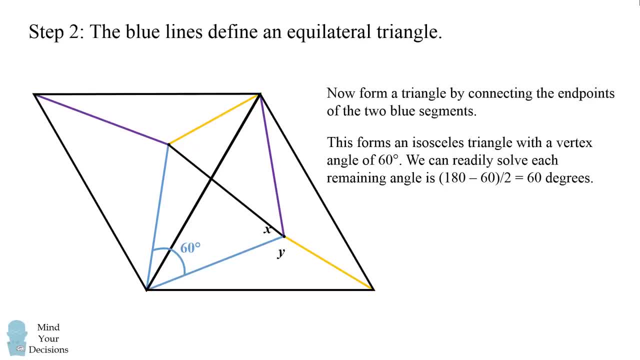 So each remaining angle will be 180 minus 60, and then we divide that by 2.. that by 2. So each remaining angle is 60 degrees. Therefore, all three angles of this triangle are 60 degrees, and so it's an equilateral triangle. So the very last. 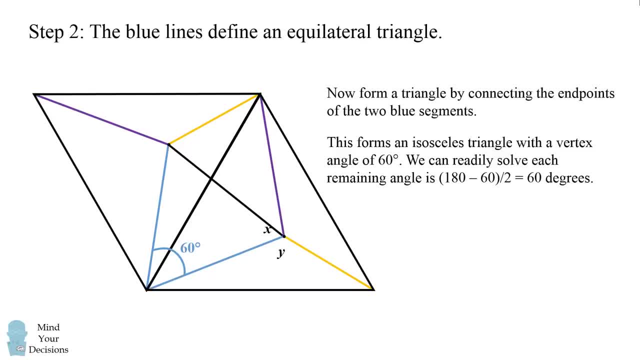 Therefore we have an isosceles triangle with the vertex angle of 60 degrees. The remaining two angles will be equal to each other and the sum of the three angles in a triangle is 180 degrees. So each remaining angle will be 180 minus 60 and 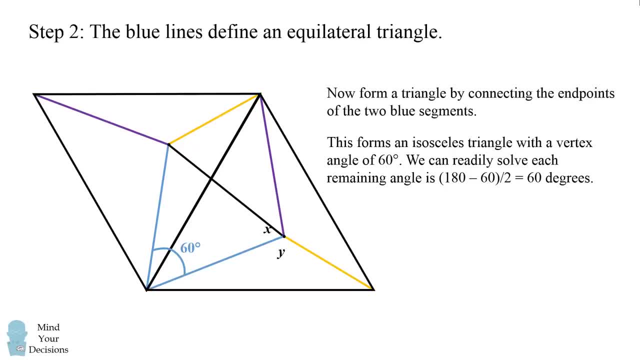 then we divide that by 2. So each remaining angle is 60 degrees. Therefore, all three angles of this triangle are 60 degrees, and so it's an equilateral triangle. So the very last side has the same length as the blue sides, So I'll color this last side in blue. 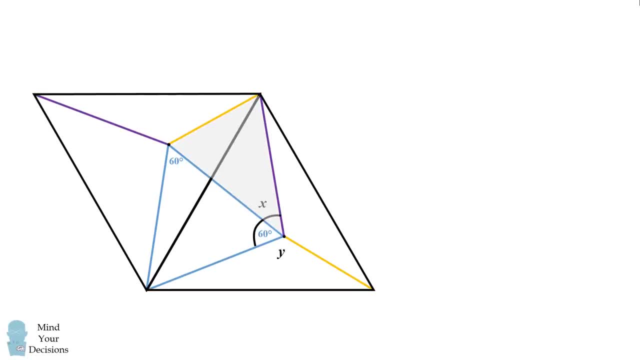 Now what can we do from here? We now have the triangle that we're looking for, with a blue, yellow and purple side, So we'll solve for the angles of this triangle. The first thing we can do is that we can solve that the angle between the purple and blue sides is x minus 60 degrees. 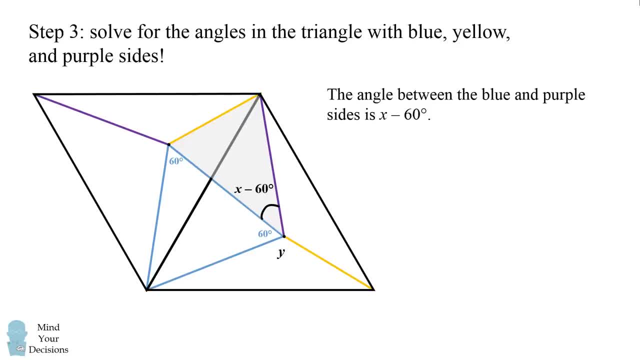 Next, we'll solve for the angle between the yellow and the blue side. This can be done because in the original triangle this angle is y. When we rotate the triangle, we know that the corresponding angle will be y and the angle that we're looking for will be y minus 60.. 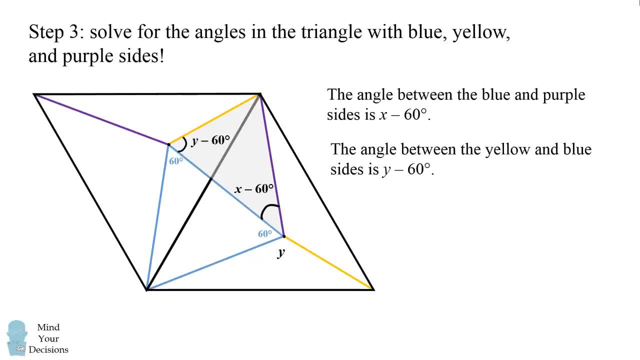 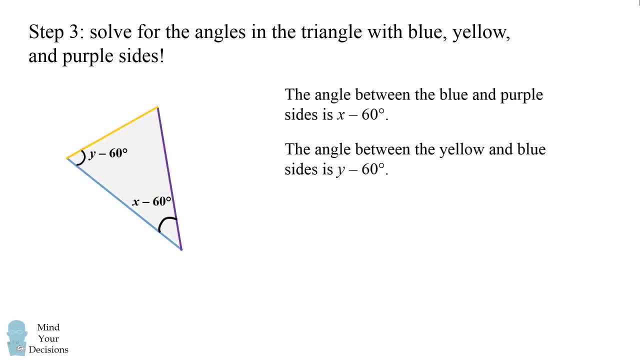 So we figured out two of the angles in this triangle and we only have one more angle to figure out. So how can we figure out this final angle? Well, the sum of the angles in a triangle is 180 degrees, So the final angle will be: 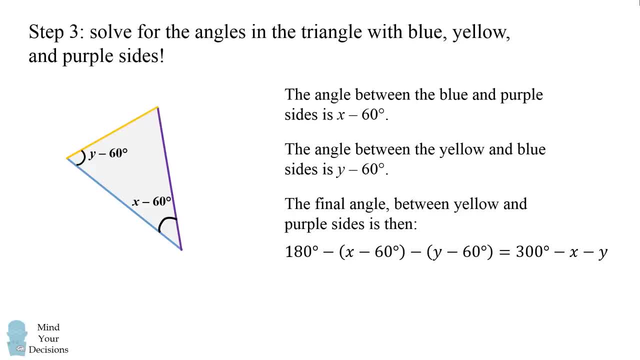 180 degrees minus each of the two angles we know: x minus 60 and y minus 60. So this will result in the angle of 300 minus x minus y, and that's the ingenious solution to this seemingly impossible problem. Did you figure it out? 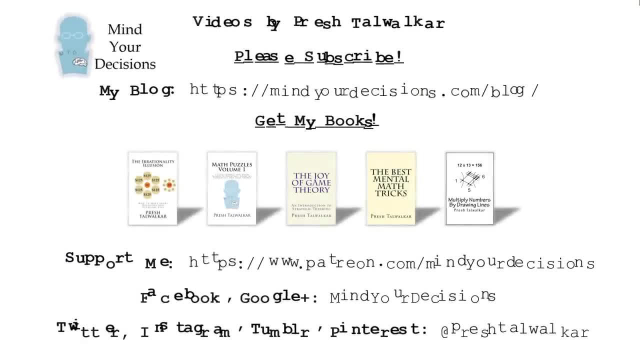 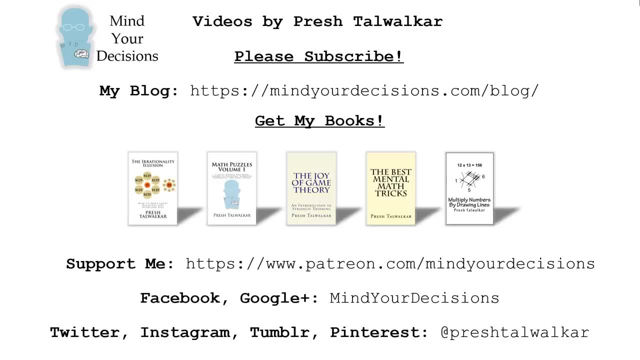 Thanks for watching this video. Please subscribe to my channel. I make videos on math. You can catch me on my blog: Mind Your Decisions. If you like this video, you can check out my books, which are listed in the video description. 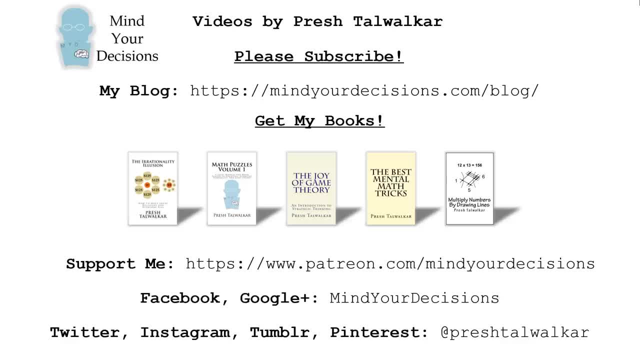 You can support me on Patreon, and you can also catch me on social media, either at MindYourDecisions or at PreshTalwalkar. 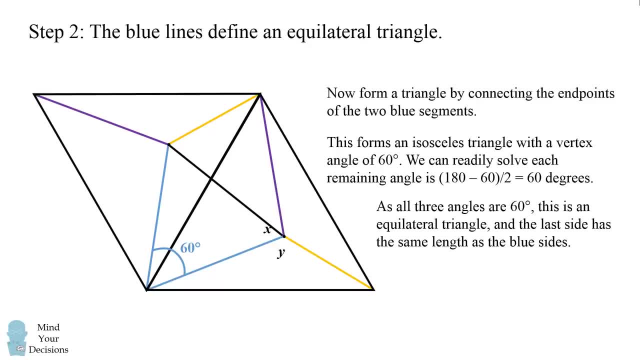 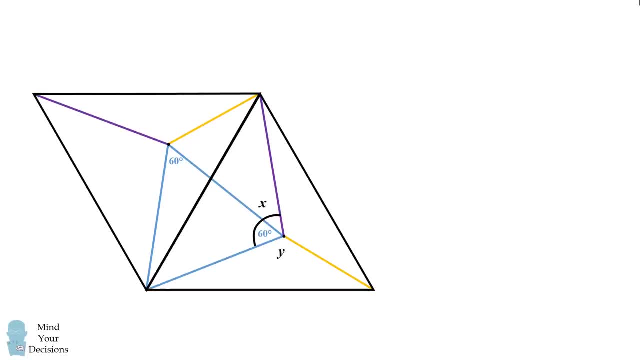 side has the same length as the blue sides, So I'll color this last side in blue. Now, what can we do from here? We now have the triangle that we're looking for, with a blue, yellow and purple side, So we'll solve for the angles of this triangle.